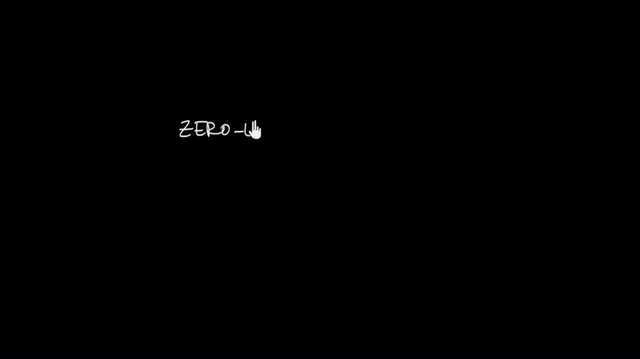 In this video we are going to look at zero order reactions. We are going to understand what a zero order reaction means. So the first thing we need to look at is: what do we mean by a zero order reaction? So what is a zero order reaction? and because we are interested in studying, 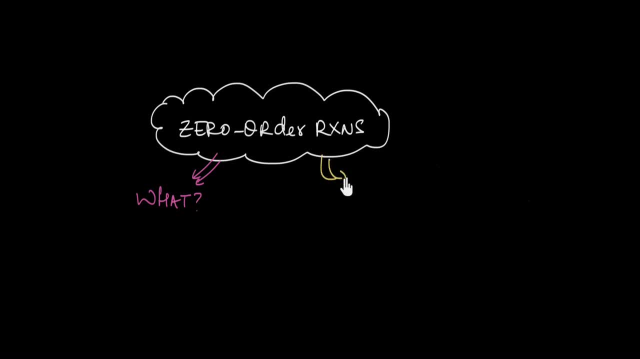 the kinetics of chemical reactions. So we are going to look at how the rate of the reaction, rate of reaction varies with different parameters for zero order reactions. We are going to look at how the rate of the reaction varies with, say, concentration and with time. 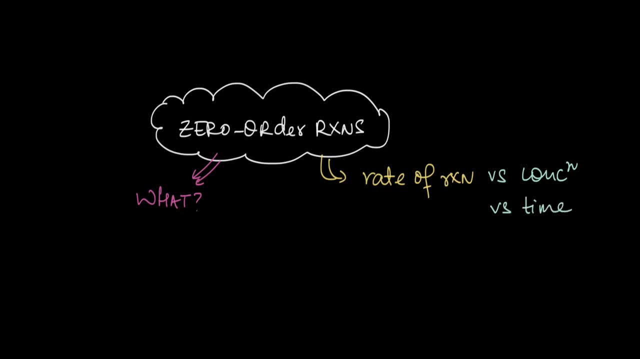 for zero order reactions. So let's start. So what is a zero order reaction? Well, if I have any chemical reaction, say A giving me products, then we know that from the rate low, we can write a reaction value 0. that is the rate of reaction we are going to write. 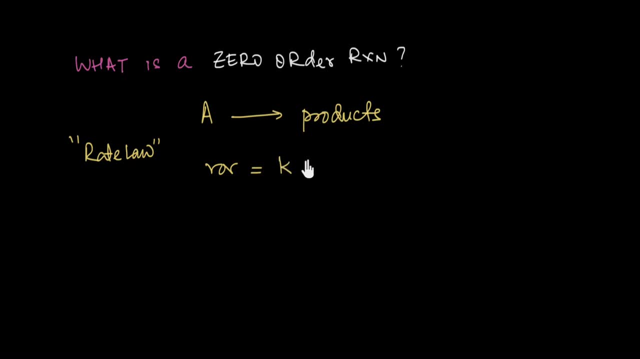 write the rate of the reaction to be equal to some constant k into concentration of the reactant raised to some power, x. now this x is an experimentally determined quantity. it's an experimentally determined quantity. you can't just look at the reaction and say what the x is. 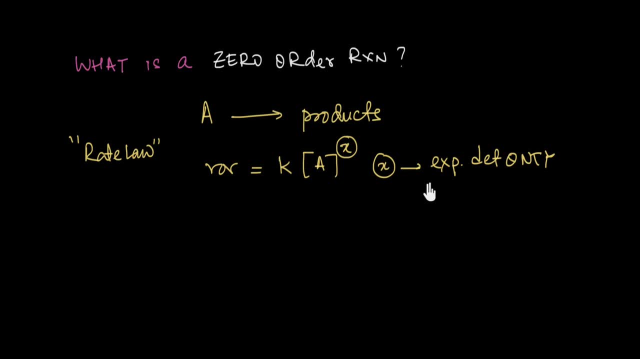 you have to figure it out experimentally and this experimentally determined quantity is called the order of the reaction. now, if it turns out, if it turns out that for this particular reaction, if the rate of the reaction can be written as k into a to the power zero, that is, if experimentally x. 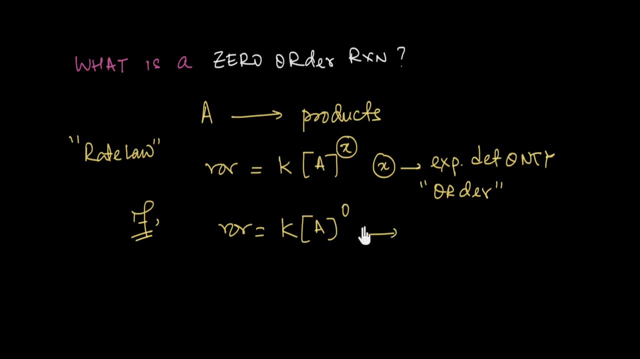 is found to be equal to zero, then the order of this reaction is zero, and so we will call it a zero order reaction. so what is a zero order reaction? a zero order reaction is nothing but a reaction. a zero order reaction is nothing but a reaction in which the whole system reaches point where each part of the reaction is zero. 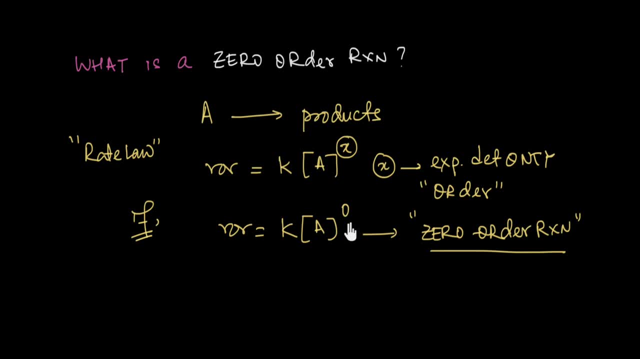 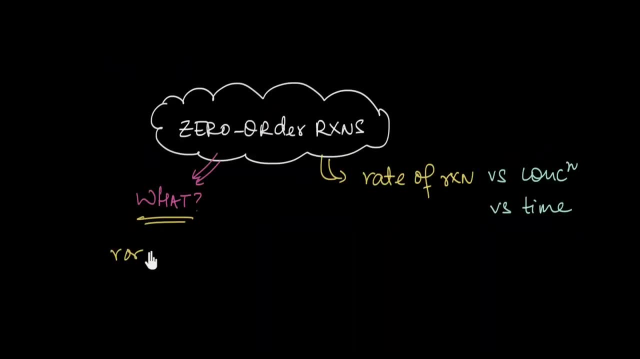 which the order with respect to the reactant has been experimentally found out to be equal to zero. So, therefore, zero order reactions are those reactions in which the rate of the reaction can be written as concentration of the reactant raised to the power zero. 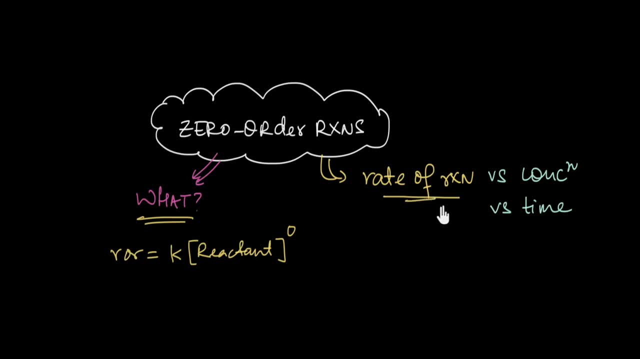 Let's now move forward and see how the rate of reaction changes with concentration and time for these zero order reactions. Let's start by looking at how the rate of the reaction changes with the concentration of the reactants. So let's say we have our hypothetical chemical reaction A giving me products, and if this? 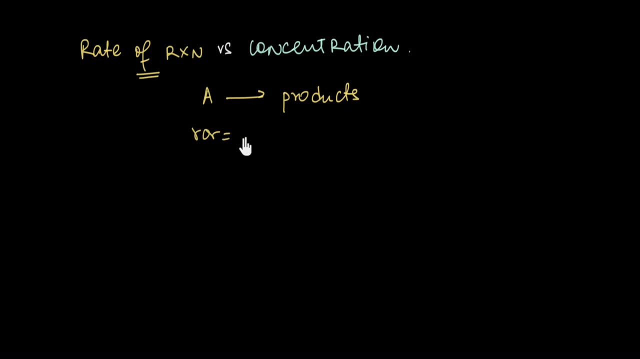 was a zero order reaction, then I can write the rate of the reaction to be equal to the rate constant K multiplied by the concentration of the reactant raised to the power zero. So what does this mean? So say, if this reaction is happening in A? 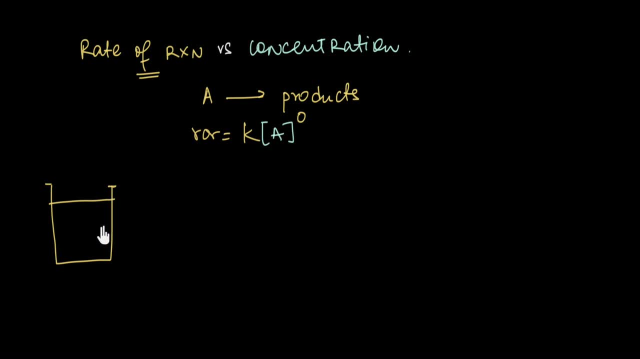 In a container and let's say that the concentration of A out here is 10 molar, Then at this instant the rate of the reaction can be written as the rate constant K multiplied by the concentration of the reactant, which is 10 molar. and because it's a zero order, 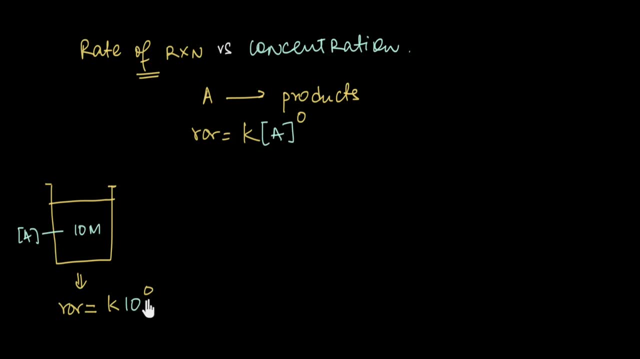 reaction so raised to the power zero, Now 10 to the power zero, is going to be equal to one right. So the rate of the reaction will simply be equal to the rate of the reaction raised to the power zero, and that will be equal to the rate constant K. 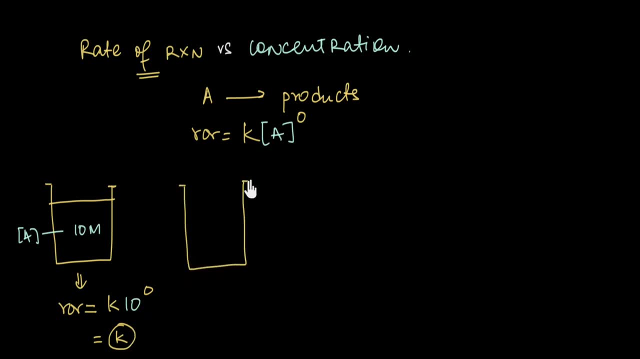 Now, instead of 10 molar, if the concentration of A was something different. if the concentration of A was 20 molar, then even out here at this instant, the rate of the reaction will be equal to the rate constant K multiplied by the concentration of the reactant, which is 20 to the power zero. 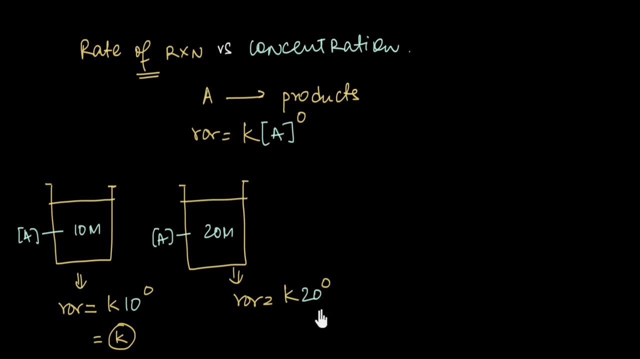 Now, even out here, 20 to the power, zero is going to be equal to one, So the rate of the reaction will simply be equal to rate constant k. so, as you can see, whatever be the concentration of the reactant for a zero order reaction, this term will always come out to be equal to one. so the rate of the reaction will be: 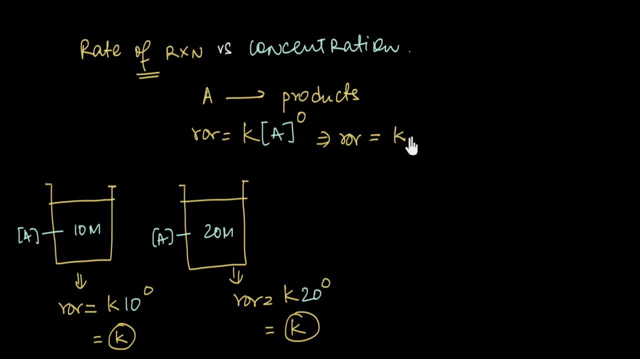 a constant, it will be equal to the rate constant k. so whatever be the concentration of the reactants, the rate of zero order reaction will always be equal to k. so if i plot a graph of how the rate of the reaction, how the rate of reaction, changes with the concentration of the reactant, 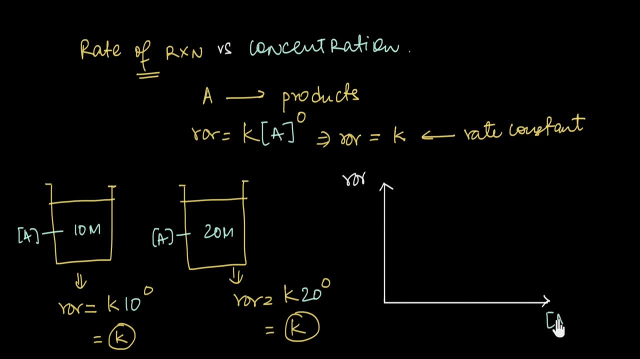 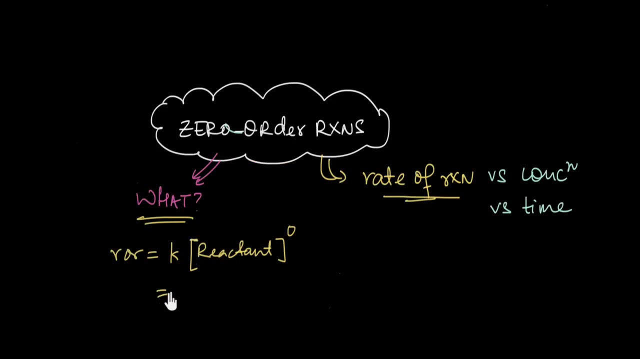 so if i have to plot a graph of rate of reaction versus concentration, whatever be the concentration of a, the rate of the reaction will always be equal to this constant value. so this will be a straight line at k. so for zero order reaction, the rate of the reaction will always be equal to the. 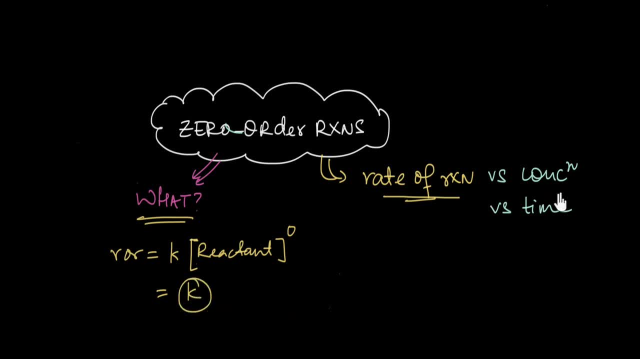 rate constant k, whatever be the concentration of the reactant. so the rate of the reaction is a constant, independent of the concentration of the reactant, of the concentration of the reactant. right, let's now look at how the rate of reaction changes with time. for zero order reactions: 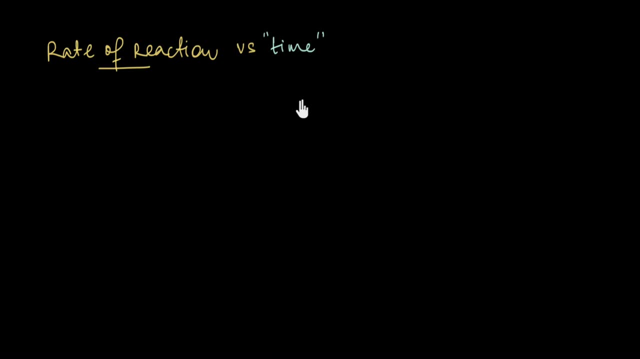 so how does rate of reaction evolve with time? for a zero order reaction? let me elaborate this a little bit further. let us say we have a reaction, a- giving me product, and let's say that we start this reaction at, say, time t equal to zero with 10 molar of a. 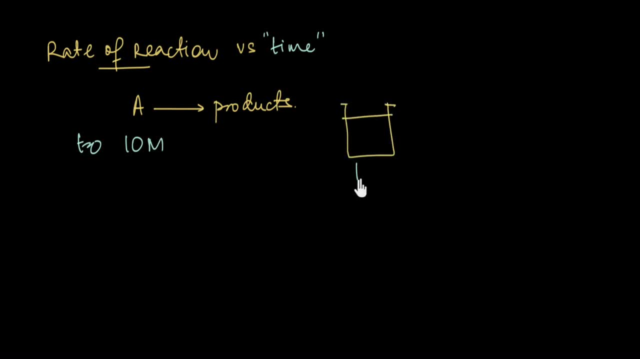 so initially, at time t equal to zero, i had 10 molar of a. now, as this reaction keeps progressing, as time evolves, some of these reactants will get converted into the products right. so after some time, say t1, the concentration of a will no longer be 10 molar. 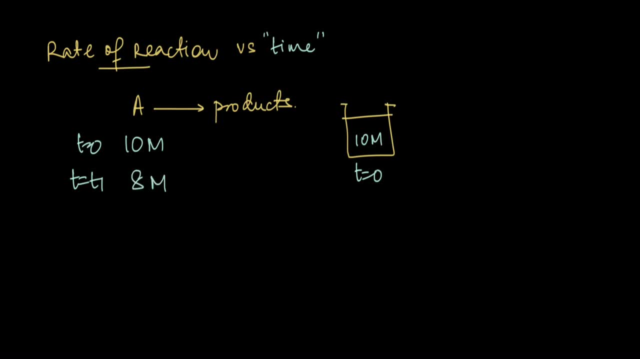 the concentration of a will drop down to say 8 molar. so after some time t1. so after some time t1, the concentration of air, let's say, drops down to 8 molar. similarly, with more passage of time, as the reaction keeps progressing, the concentration of air will drop down further and say it drops down. 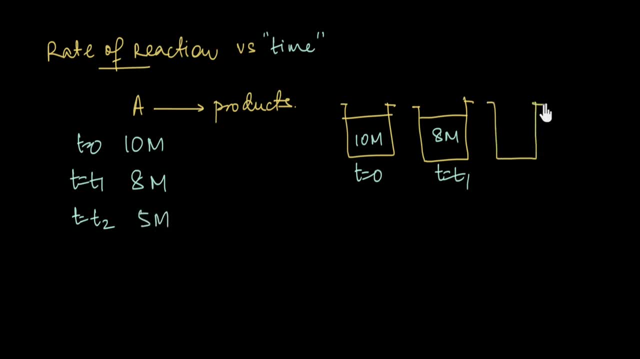 to say 5 molar, at say, time t equal to t3. so at time t equal to t3, the concentration of a drops down to 5 molar. so now, if i want to plot a graph of how the rate of reaction changes throughout the course of this reaction, so how the rate of reaction changes with time, what would that? 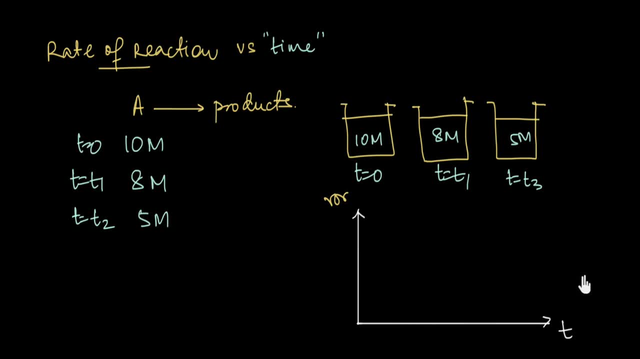 graph. look like you can pause the video and see if you can come up with the answer. well, with time, the concentration of the reactant keeps gradually decreasing, right. however, since this is a zero order reaction, since rate of the reaction is k into concentration of a to the power 0, so whatever. 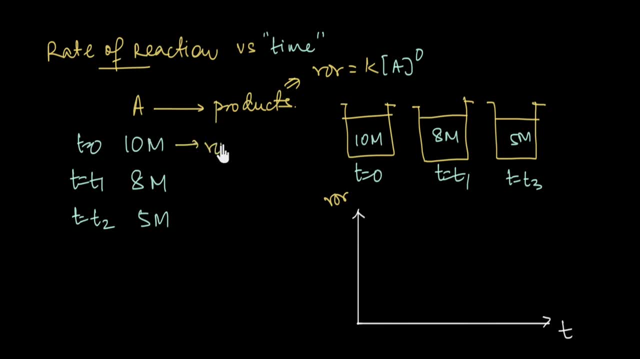 be the concentration of the reactant. the rate of the reaction will always be equal to the rate constant k, right? so it doesn't matter if the concentration of a is 10 molar or 8 molar or 5 molar. the rate of the reaction will always be equal to the rate of the reaction of the reactant. 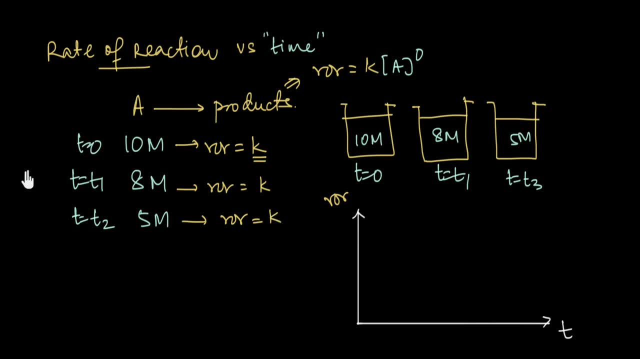 and the rate constant k. so now, if we check it with respect to time, then initially the rate of the reaction was equal to k and now, after some time, t1, it will still remain k and it will forever remain k. so over time in zero order reactions the rate of the reaction doesn't change and it keeps constant. 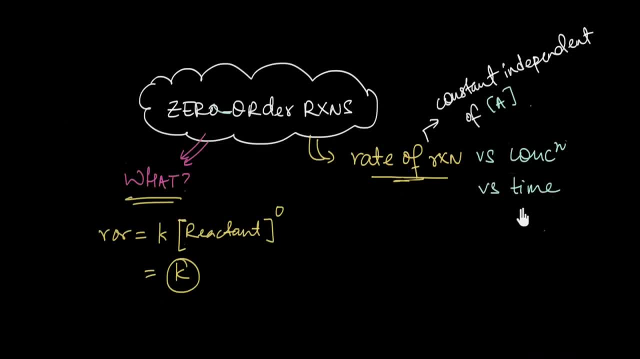 throughout the course of the reaction. so with time over the course of a zero order reaction, the rate of the reaction doesn't change and it is constant throughout the course of the reaction. now, if you have stuck around till now, i'd like to add that zero order reactions actually do not make much. 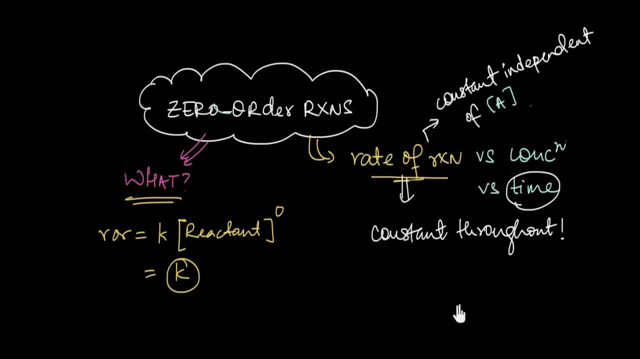 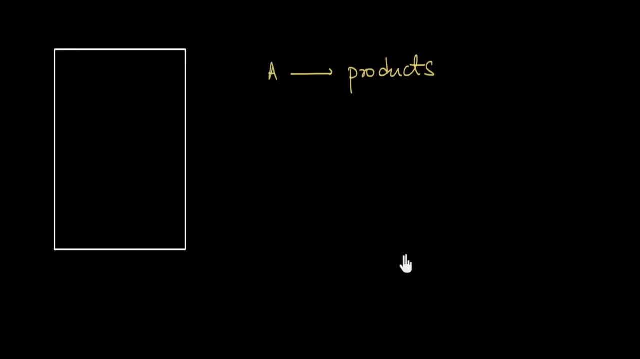 sense. in fact, to be honest, zero order reactions kind of go against everything that we have learned till now. let me show you how now. we have always maintained that a chemical reaction happens when the reactant molecules collide against each other. now, if the reactant molecules are few and far between, then the probability of these collisions will be lower. 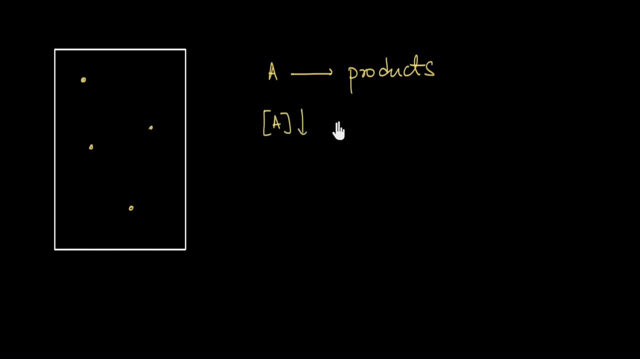 so when the concentration of the reactant molecules is low, the rate of the reaction should be low. and if the concentration of the reactant molecules is high, then the probability of these reactant molecules colliding against other each other will drastically increase. and so if the concentration 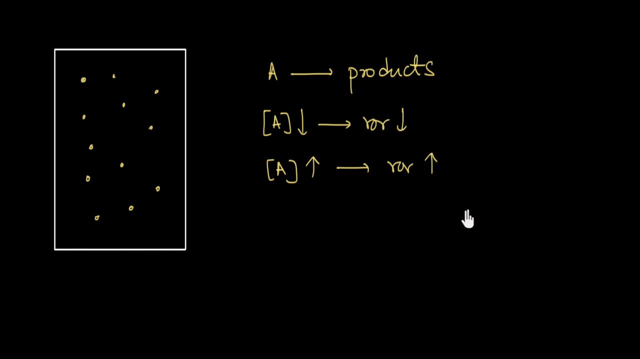 of air increases, then the rate of the reaction should increase, right? however, zero order reaction totally does not fit into this picture. for a zero order reaction, the rate of the reaction is independent of the concentration of the reactant, so it doesn't matter if i increase or decrease. 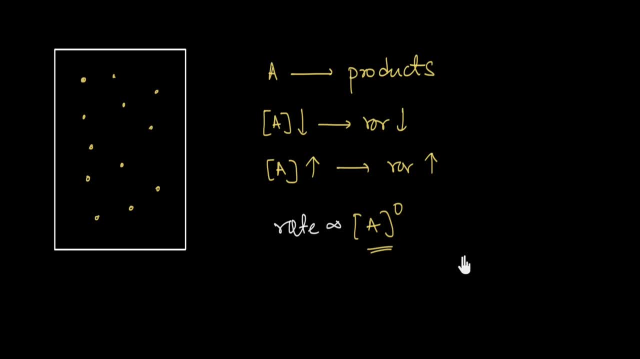 the concentration of the reactant, the rate of the reaction won't change. wow, are such reactions even possible? let's see. let's take a look at this reaction, the decomposition of n2o into n2 and o2. now, if we carry out this reaction in the gaseous phase, so if we like, simply take a container and 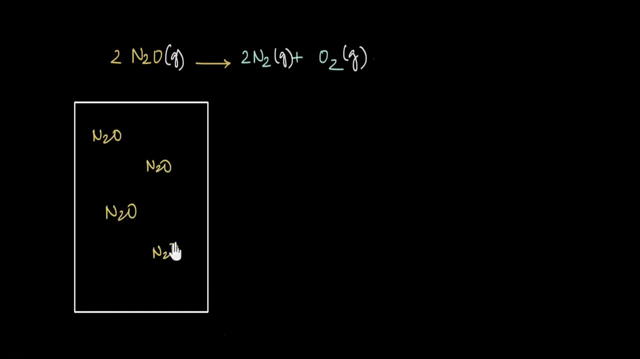 fill it with n2o molecules, then these n2o molecules will collide against each other and some of the old bonds will get broken down and some new bonds can get formed. so some of these collisions will lead to the formation of n2 and o2. now, if you think about it, if i increase the concentration of n2 out here, 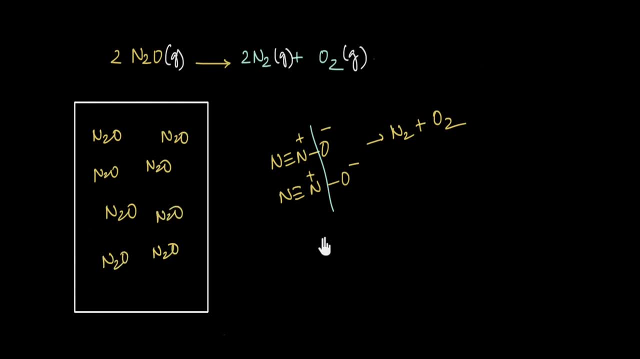 the overall number of collisions between the reactant molecules will increase, so the probability of successful collisions will also increase. so the rate of the reaction should increase, right? so if i increase the concentration of n2o, the rate of the reaction should increase. now, experimentally, the rate of this reaction has been found out to be equal to the rate constant k. 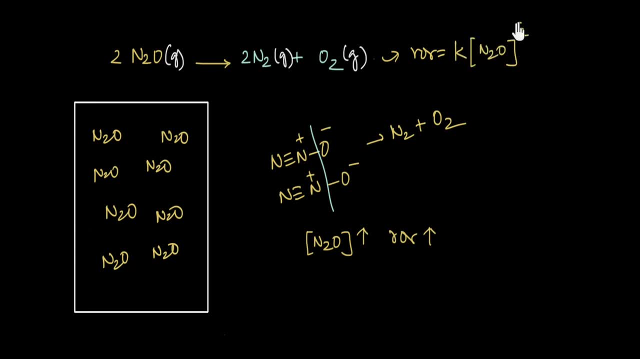 multiplied by the concentration of n2o to the power 2.. now, this is nothing contradictory. even this is just a very simple example of the reaction of n2o. and if i increase the concentration of n2o, then the rate of the reaction will increase, and if i decrease the concentration of n2o, the rate of the 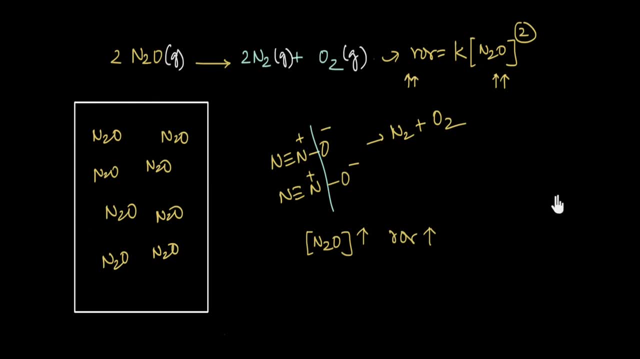 reaction will decrease. nothing surprising out here, right? however, this is a very slow reaction and instead of carrying out this reaction in this way, it is generally carried out in the presence of a catalyst like nickel. so instead of simply taking it in a container and letting the collisions happen, 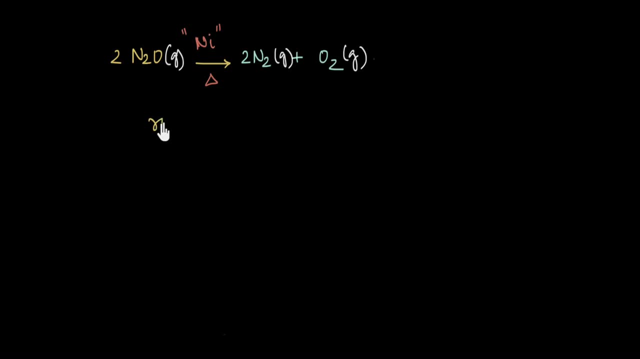 this reaction is taken out of the present of nickel, and then the reaction is taken out of the present of n2o, and then the reaction is taken out of the present of n2o, and then the reaction is carried out in the presence of a catalyst like nickel. so if you take this reaction in the presence 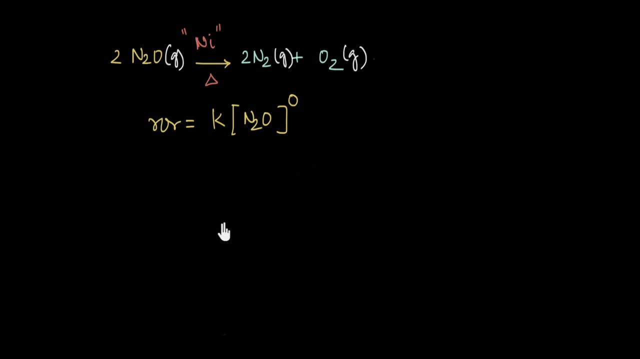 of nickel. then experimentally, the rate of the reaction is found out to be equal to the rate constant k multiplied by the concentration of n2o to the power 0. so this becomes now a zero order reaction. so what exactly is happening out here? let's see. 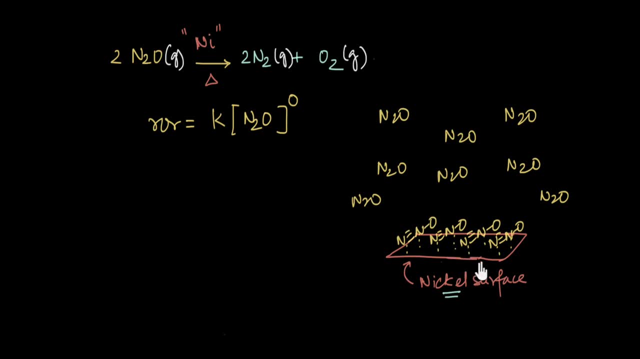 Now, in the presence of nickel, the n2o molecules get absorbed at this nickel surface. in other words, they use some of their electrons to form bonds with this nickel molecule metal. so because they use some of their electrons to make new bonds, so their old bonds gets weaker. 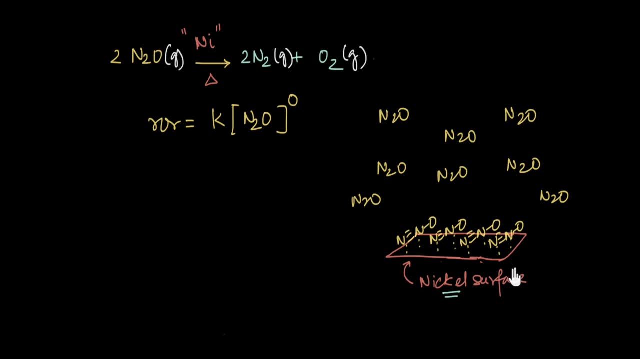 and therefore these n2o molecules that are absorbed at the nickel surface. these n2o molecules, on collision, can break the bonds much more readily, leading to the formation of n2 and o2. so this is how nickel catalyzes the decomposition of n2o. however, having said that, as you can see the rate, 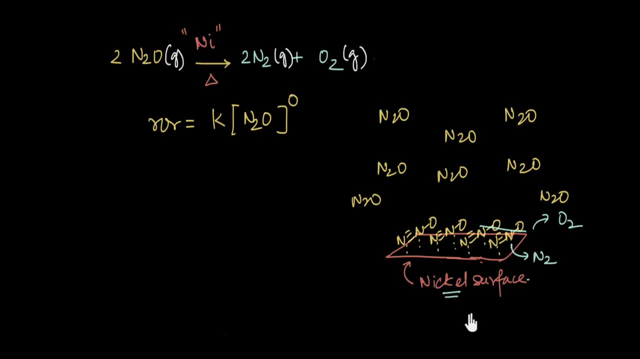 of n2o is quite relatively limited by the surface area of nickel that's available for adsorption. now, generally, the number of gaseous molecules that we have is much, much greater compared to the available adsorption sites. so once these adsorption sites are filled- which happens pretty quickly- these 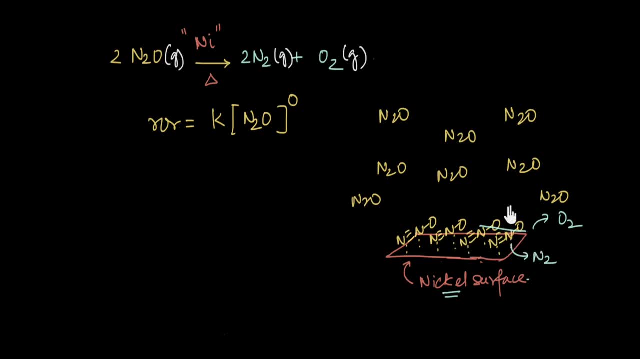 unabsorbed n2o molecules have to wait for some of these reactions to happen, and only when this sites get freed up. only then they can get absorbed. So in this scenario, if I keep increasing n2o molecules, by Kendrick's Law these N2O molecules are found to be very likely to absorb nickel. 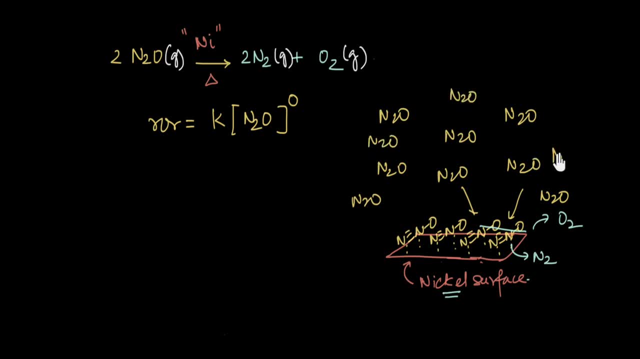 only then they can get absorbed. increasing the concentration of N2O: this is not going to lead to a consequential increase in the rate of the reaction, right? so if I increase the concentration of N2O, there is going to be no change in the rate of reaction. 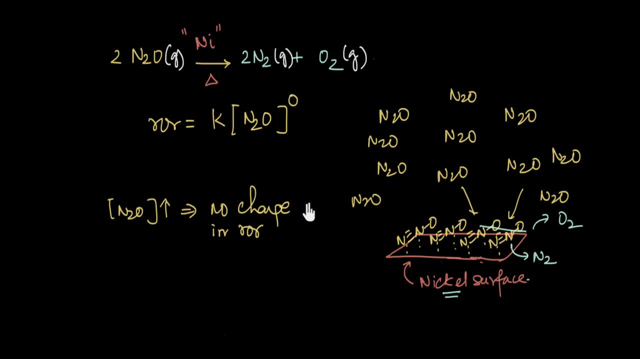 under these circumstances. so that is why, under these conditions and the rate of the reaction is zero order with respect to N2O. now, a quick note that I'd like to add out here is that, as this reaction keeps happening as more and more N2O, 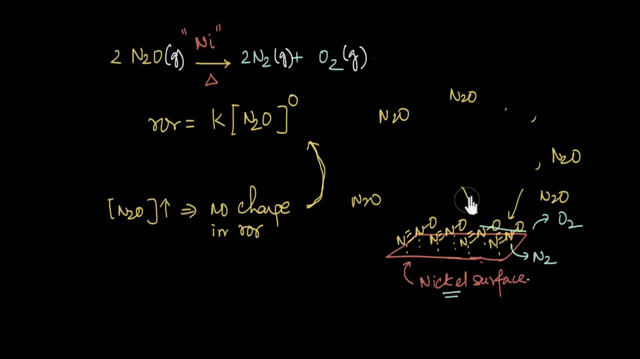 molecules convert into N2NO2, then ultimately, it might so happen that the number of N2O molecules are not in excess compared to the adsorption sites. so in such a scenario, the reaction will no longer be zero order and will revert to some other order. so what I am trying to say is that in reality, we actually 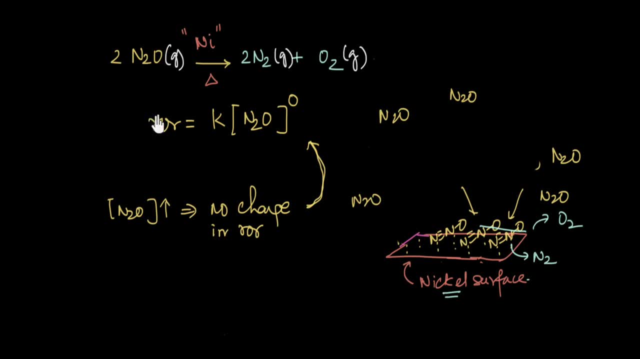 cannot have a reaction that is not going to lead to a change in the rate of reaction. that's like a hundred percent zero order all the time.